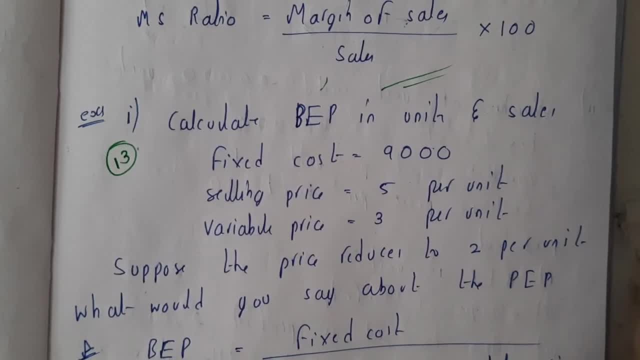 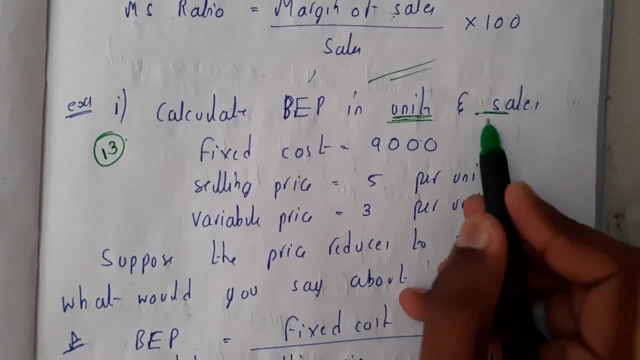 problems guys, so that you'll be having a clear idea. Okay, so the first problem is given in this way: calculate the BEP break even point in units and sales? So you give in the question it's: you need to calculate in units and sales. I hope everyone remembers the formula of units. 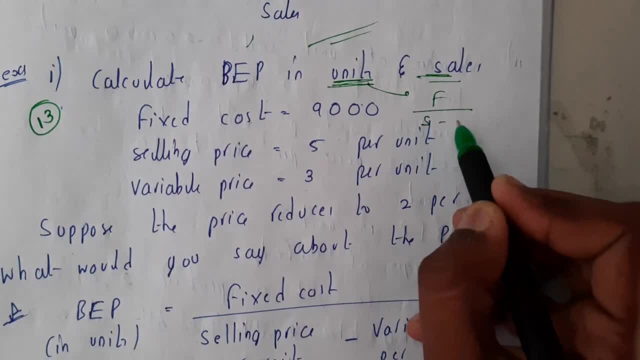 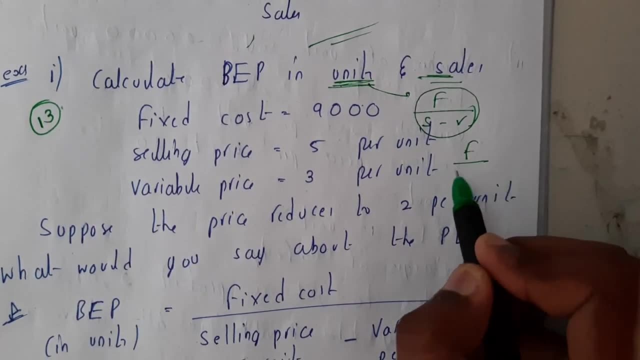 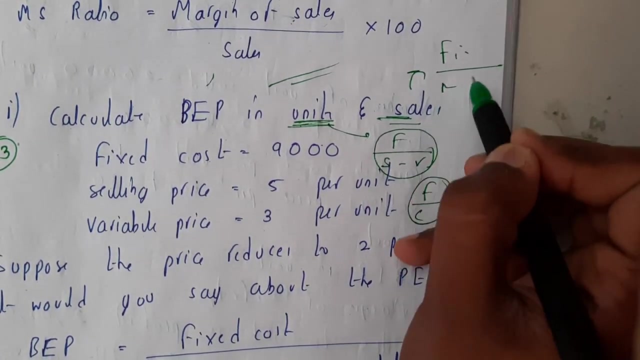 that is nothing but fixed cost by sales: my sale selling price minus variable cost. So this- or you can also write it as f by that- is nothing but fixed cost by contribution cost. Okay, similarly, sales can be written as a fixed cost by PV ratio or fixed cost, sorry- fixed cost by contribution. 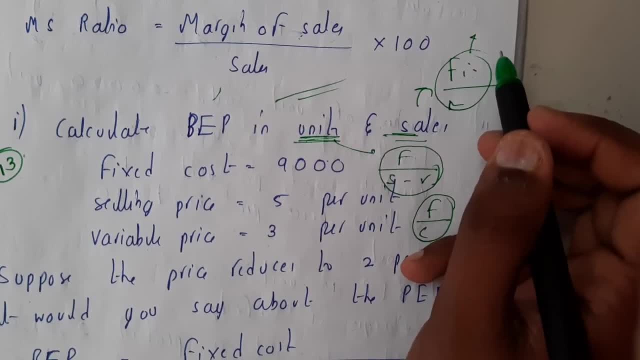 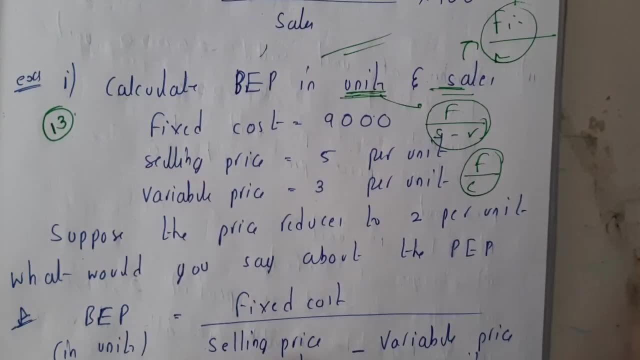 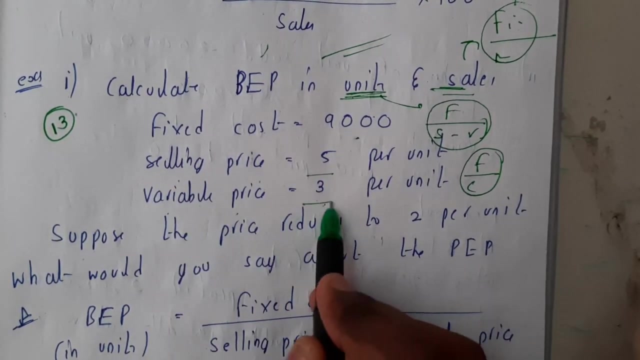 into sales or fixed cost By sales minus variable into sales. Guys, we'll be discussing one. you'll be using one, only one formula, guys. it's really simple, don't worry. Okay. so in the question he gave fixed cost equal to nine thousand, selling price is five and variable price is three. Okay, so then suppose the price. 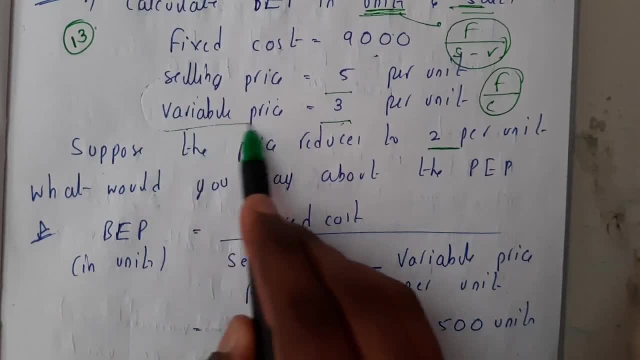 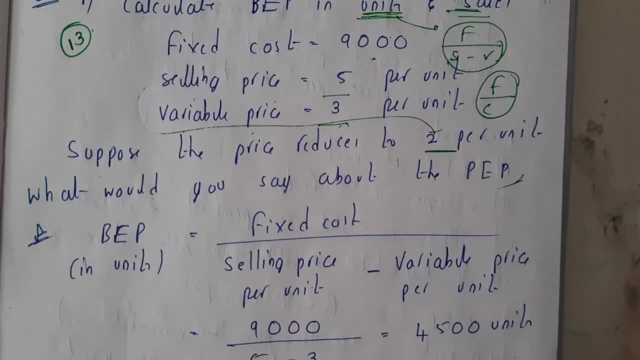 reduced to two. So he's selling saying that the selling price reduced to two per unit, What would be? what would you say about the problem? What will be the final result, whether it is in profit or in loss? So we all know the formula. in units, guys, that is nothing but fixed cost by selling price per. 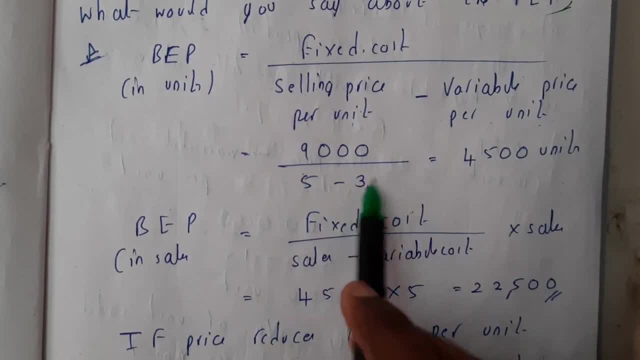 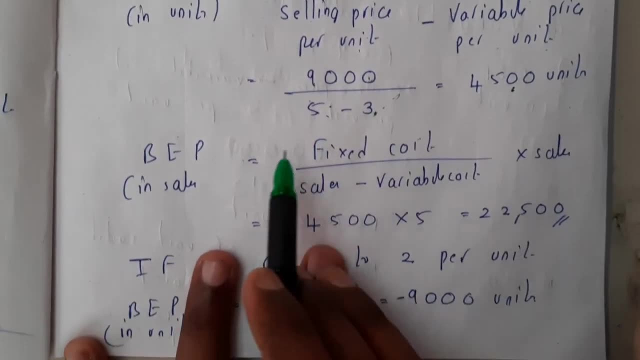 unit minus variable price per unit. So nine thousand by five minus three. So five minus three is two. So we got two by nine thousand is nothing, but sorry. nine thousand by two is nothing but four, five, double zero. So we got four, five, double zero units. Okay, so now we are done with units. So the 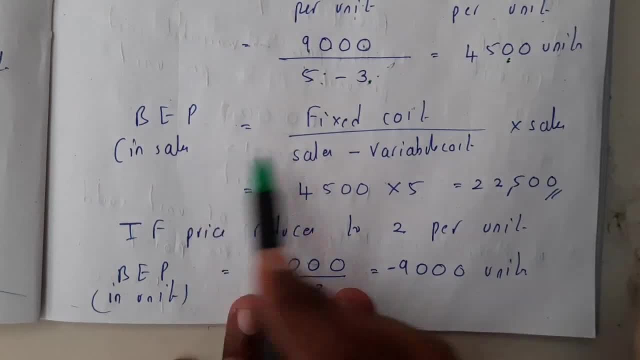 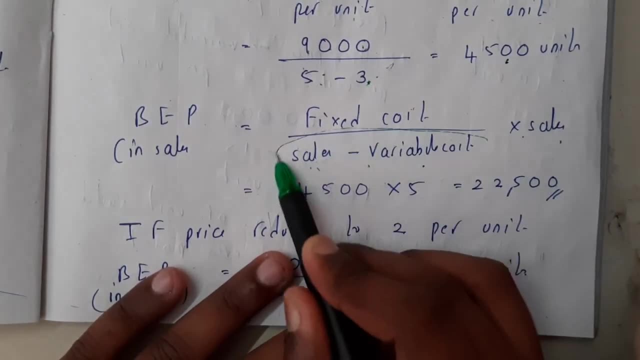 sales, the sales of the congested or the expanded. formula is this, guys: fixed cost by sales minus contribution into sales. So if you remember this formula, this is nothing but contribution. So contribution by sales is a nothing but PV ratio. So BEP is nothing but fixed cost by PV ratio. 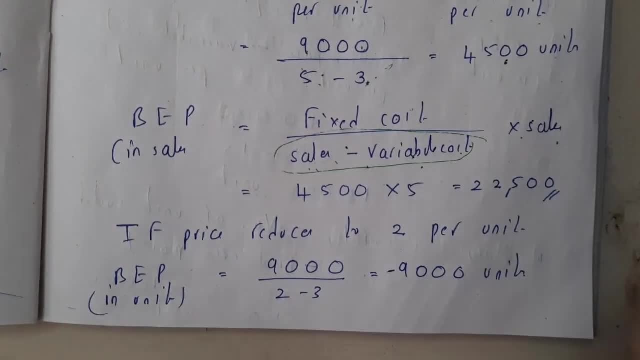 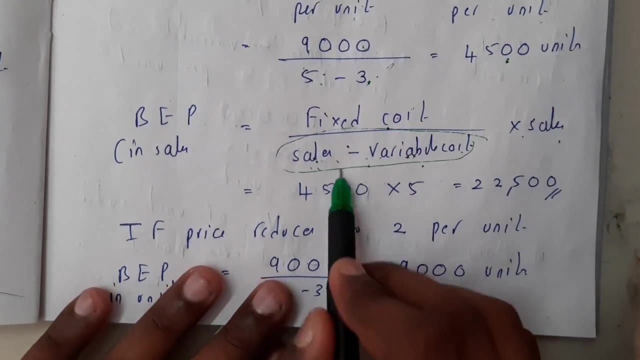 So just by remembering this formula you can derive all the formulas, guys. Okay so, fixed cost: we already know it is nothing but nine thousand, and we already have the value sales minus variable: that is nothing but two. Nine thousand by two is four thousand five hundred into sales Sales is. 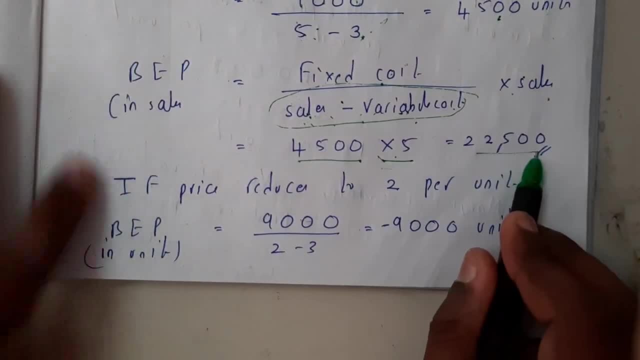 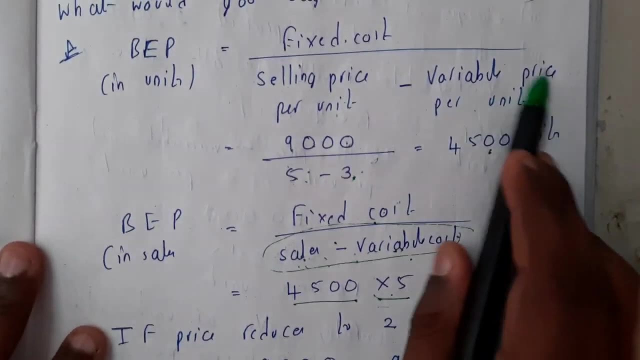 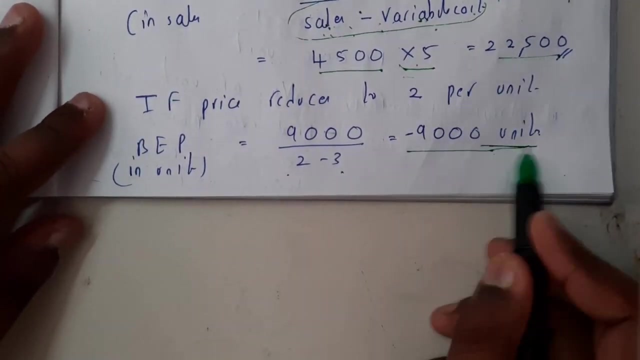 five, right selling price, So five. So we got twenty. two thousand, five hundred. Okay. so he also told us of a variable, sorry selling price instead of five. place to nine thousand by two minus three, So we got minus nine thousand units. So you are losing nine minus nine thousand units, guys. So that could. 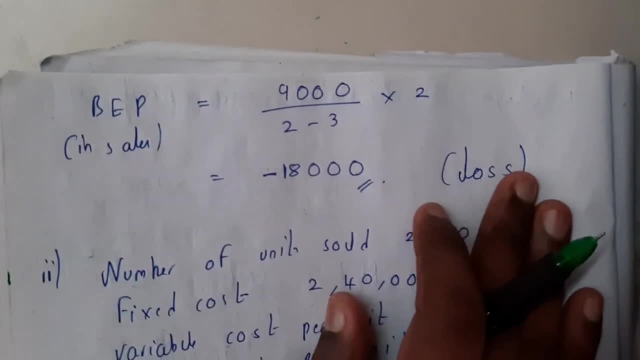 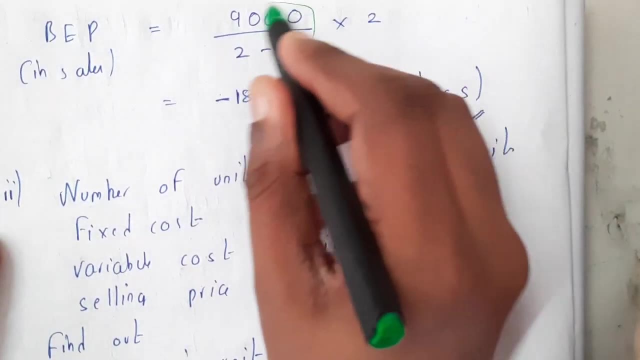 be an issue, right? So that's loss. So similarly, if you want to calculate in terms of cash, this will be in reverse format. I hope everyone knows that. So nine thousand we got again. So write the same answer: guys, Here you got minus nine thousand right directly, So into two that is nothing but. 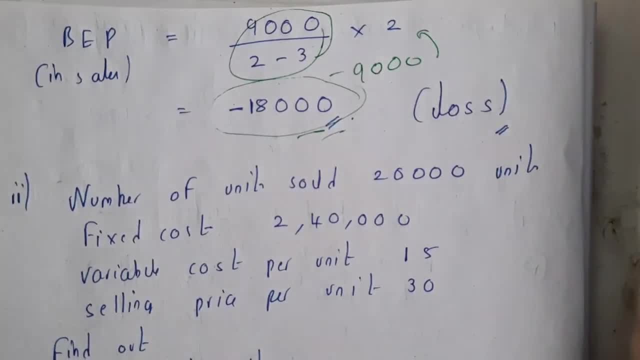 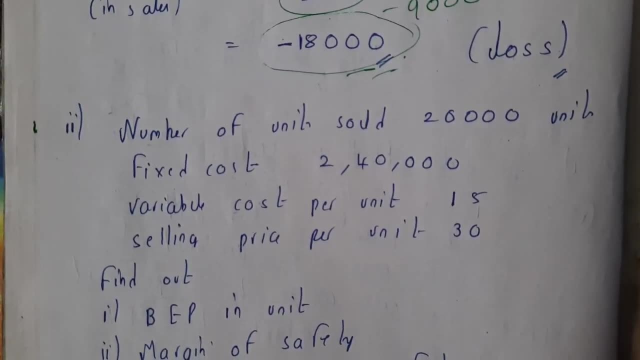 minus one, eight, double zero, So you're using this much of cash, guys. So I hope everyone got a small idea on this problem. So, if possible, take a piece of paper and solve it again, guys, So that you'll be having a clear idea. Okay, So now let us go through the second problem. So in this, the 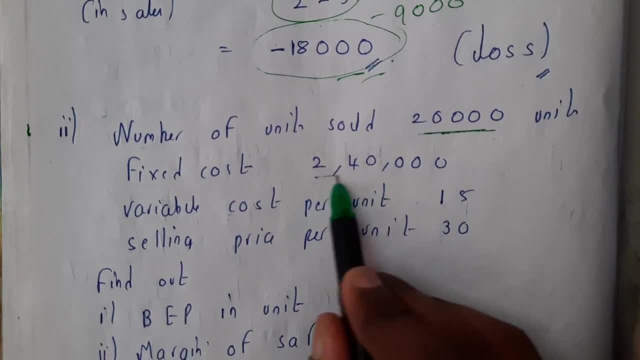 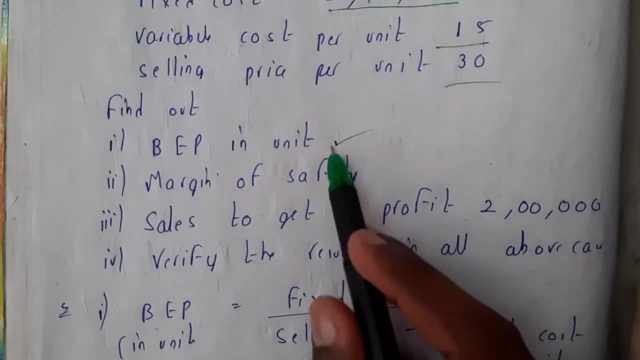 number of units sold? he gave twenty thousand. Fixed cost is two lakh forty thousand. Variable cost is fifteen and selling cost is thirty. Okay, he asked us to find the BEP. that is nothing but break-in point in units itself and marginal safety and sales to get to the profit two lakhs. 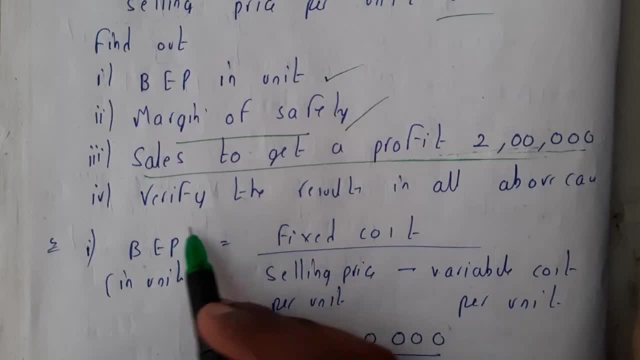 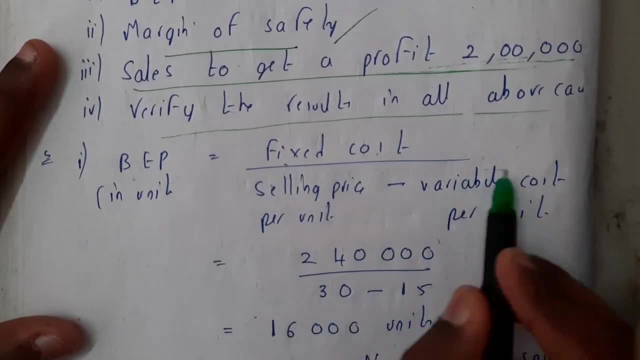 So now here he gave that we need to get a profit of two lakhs and verify the result in all The above cases. Okay, So the first thing is unit. I hope everyone knows fixed cost by selling price per unit minus variable cost per unit. Fine, So you will be just solving it So by 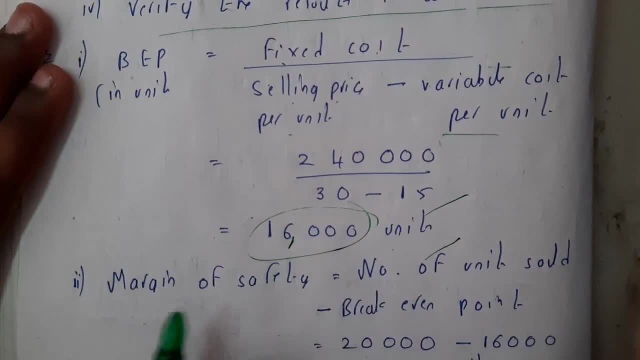 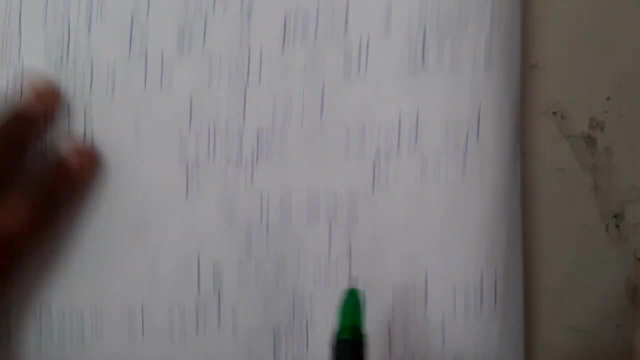 substituting it we got sixteen thousand units are the selling units which we are selling. So what is the margin of safety? means how many units we are having with us after selling. So initially we are having twenty thousand. So we, at sixteen thousand, we will be in no profit or no loss yet. 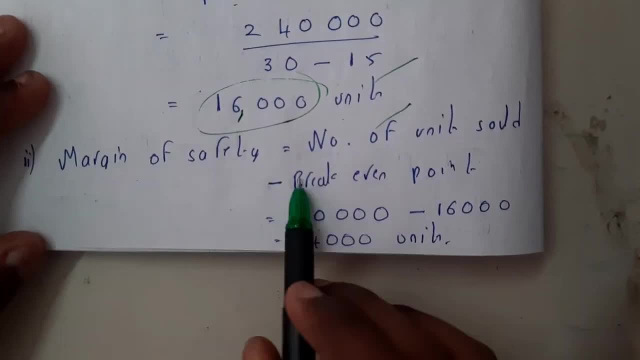 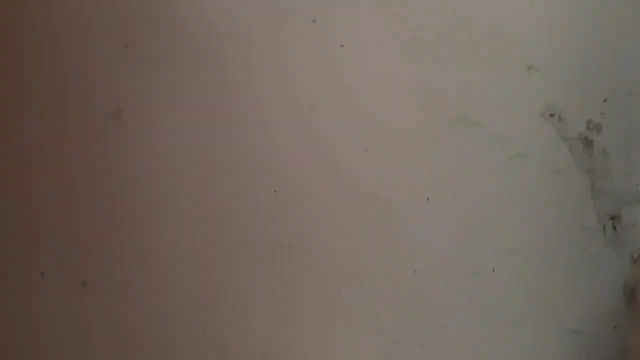 So what are the left out things? So that is nothing but your margin of safety. So margin of safety is the number of units sold minus break-in point. So twenty thousand minus sixteen thousand, that is equals to four thousand. So if you sell those four thousand units you will get a profit in that. 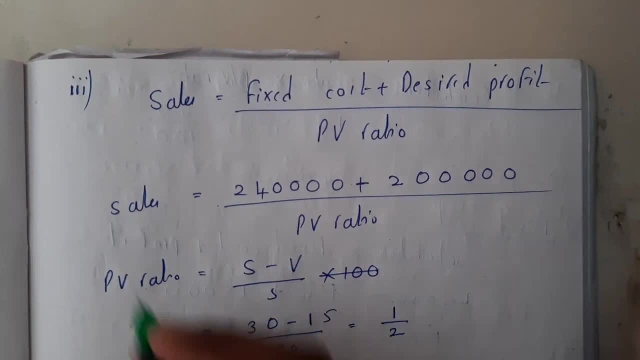 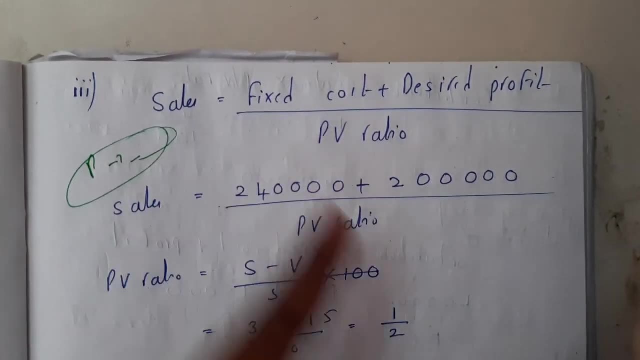 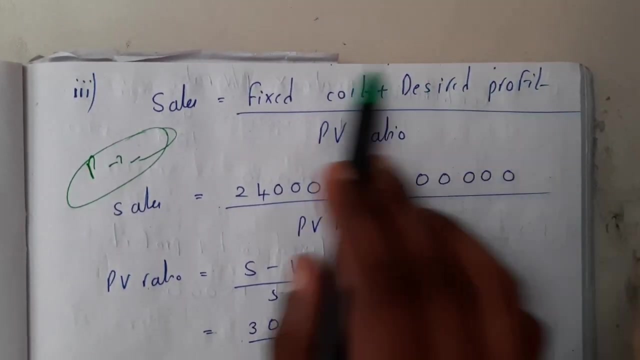 way, Fine, Okay, So I told you that we need a profit of two lakhs, Right, So for that. this is a small formula, guys. So this formula Is that- I hope everyone noticed that- Okay. So sales is equals to fixed cost plus the desired profit by PV ratio for any kind of thing he gave, even if we asked.